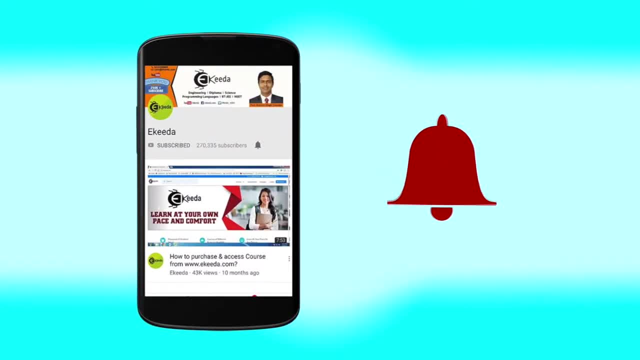 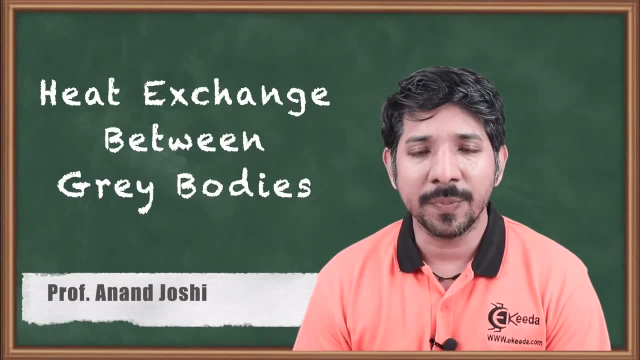 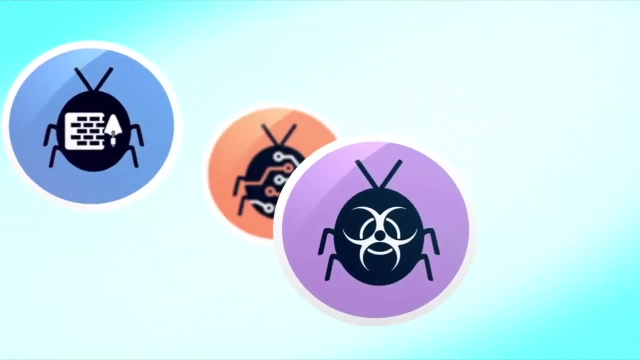 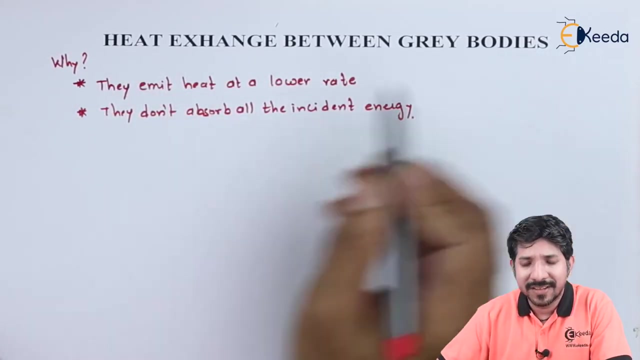 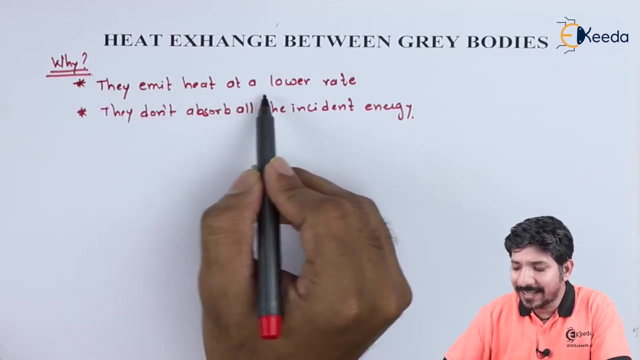 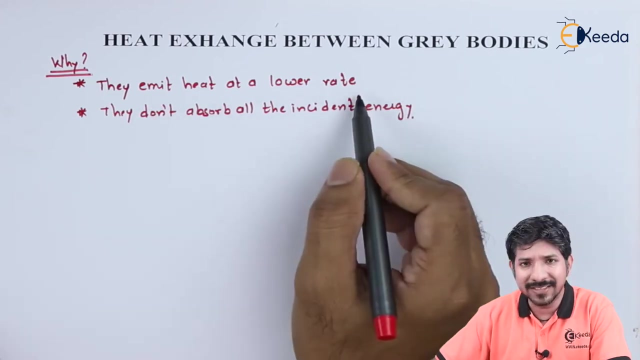 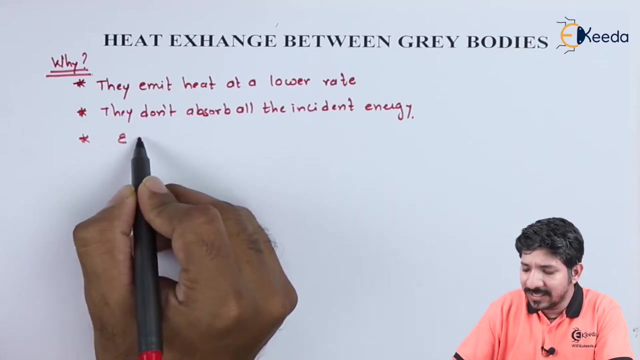 Click the bell icon to get latest videos from eKIDA. They emit heat at a lower temperature. That is the first thing. Second is they don't absorb all the incident energies. Now, these are the two of the things which we need to consider, And obviously we know that, in case of a grey body, the value of emissivity is same as the value of absorptivity. 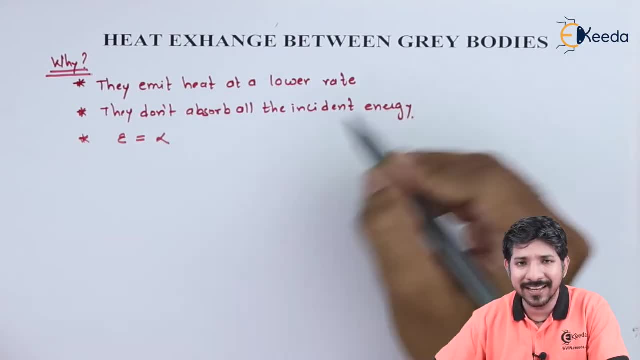 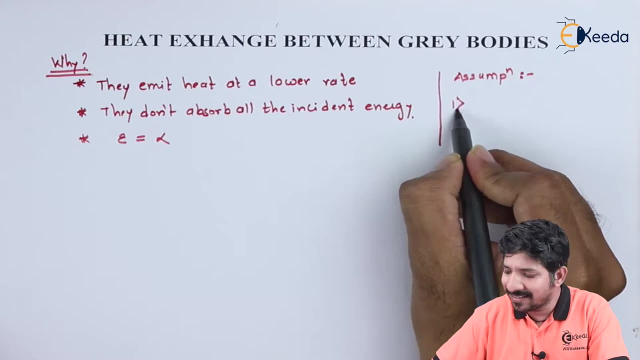 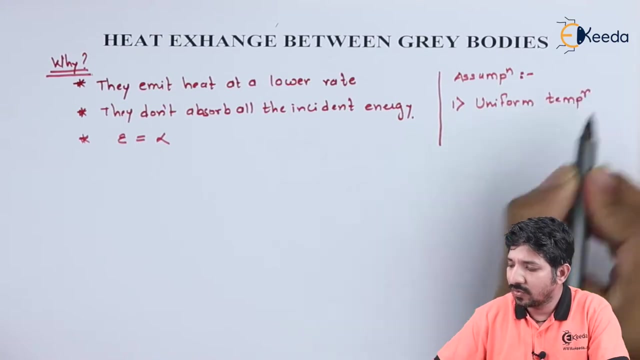 So, due to this thing, we are going to consider the heat exchange between the grey body. That is one of the reasons, And in that we are going to assume that my entire surface is is kept at a uniform temperature. So that is my first assumption. Then second one is: obviously the radiation is in the form of diffuse radiation. 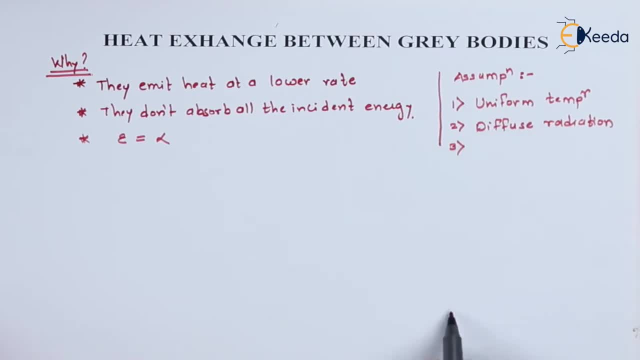 So I hope all of you understand what do you mean by diffuse radiation, The radiation which are coming onto the body. they may get reflected at certain angle. So that kind of radiation is what we call as a spectral radiation. But in this case we are going to assume that we don't have spectral radiation. 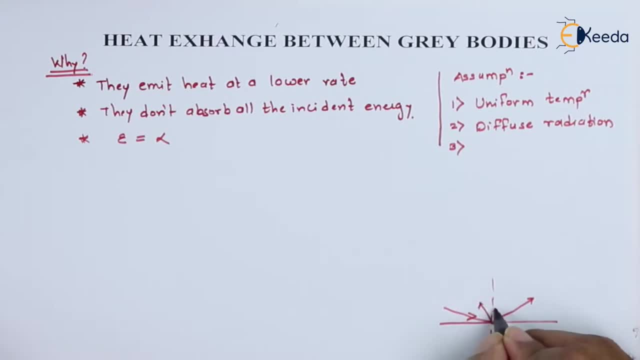 But in fact we are going to have a diffuse type of radiation. So means the radiation may take place in all the hemispherical direction. So that is one of the assumption, That is, the radiation is a diffuse type. And then third one is the opaque body. 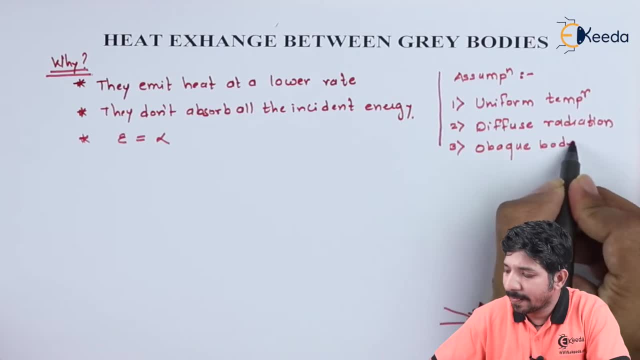 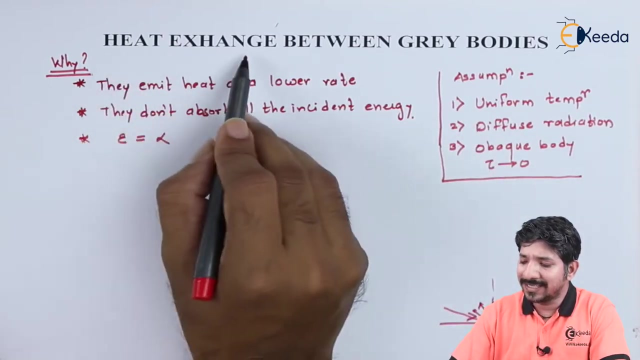 So what do you mean by the opaque body? That the transmissibility associated with that is always zero. Now, with these three main assumptions in our mind, we can talk about the heat exchange between the grey bodies. Now, along with that, we need to also discuss about two properties. 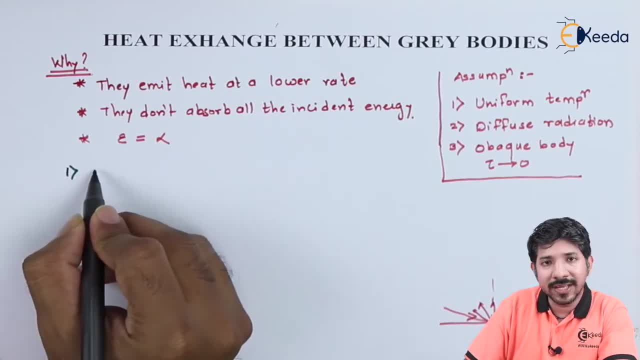 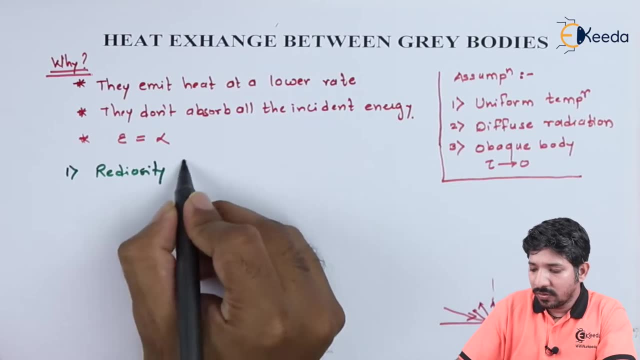 We have already discussed the two properties, but we need to go for the recap of the same. So the first one is radiocity, which is indicated by J. Now, what is radiocity? Now, radiocity is nothing but the amount of energy. 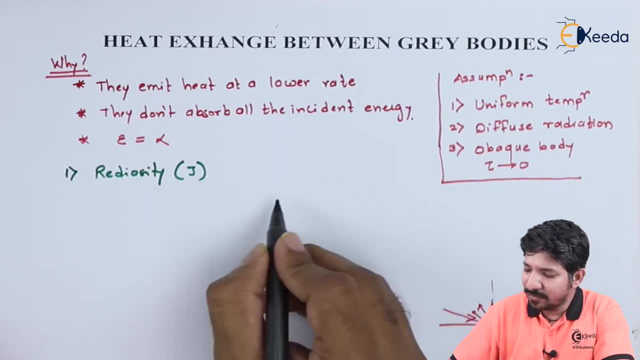 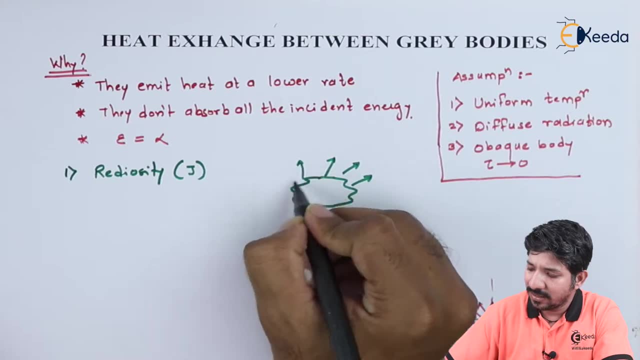 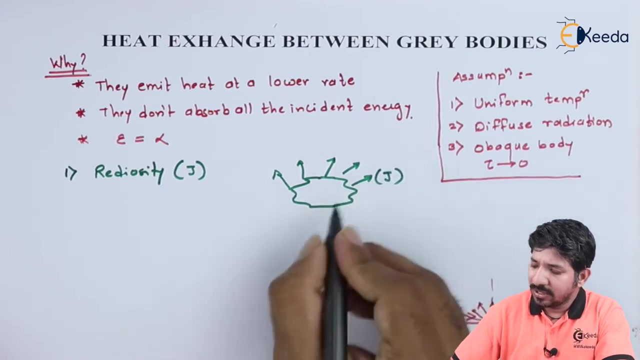 So instead of writing it, I can simply explain. Suppose this is the body, Then the amount of energy radiated by the body in the hemispherical direction, let us say G Now the amount of energy radiated in the hemispherical direction per unit time. 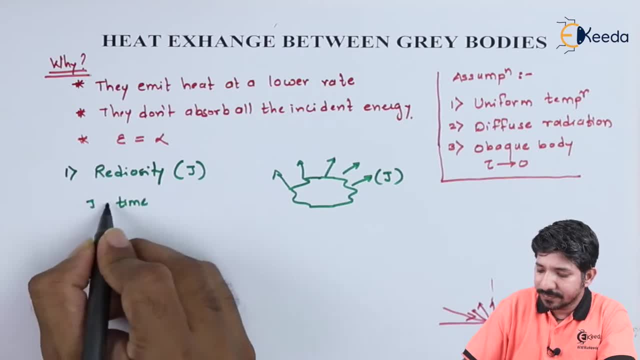 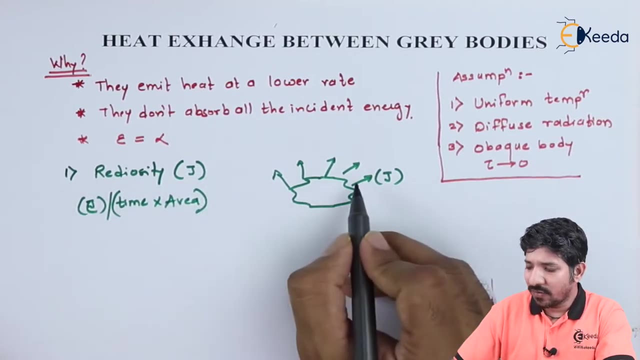 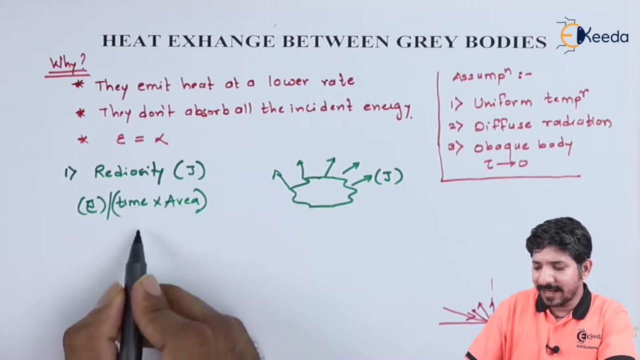 So this can be expressed as the energy, let's say E per unit time and per unit area. So now this also can be given for all the wavelengths. So again, the four things that one must understand: time, area, wavelength and direction. 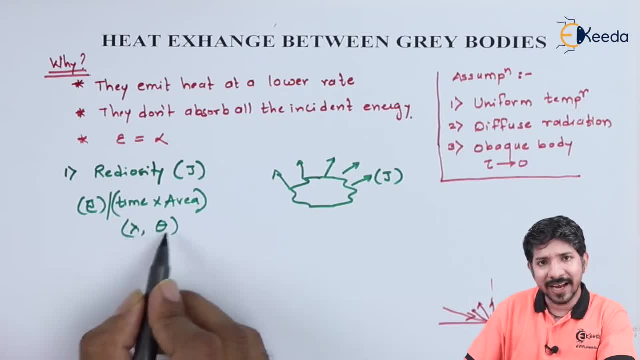 So again we are going to consider that, for all wavelengths and for hemispherical direction, the amount of energy that is radiated per unit time, per unit area. This is all about the radiocity. Again, the value of J comprises of two things. 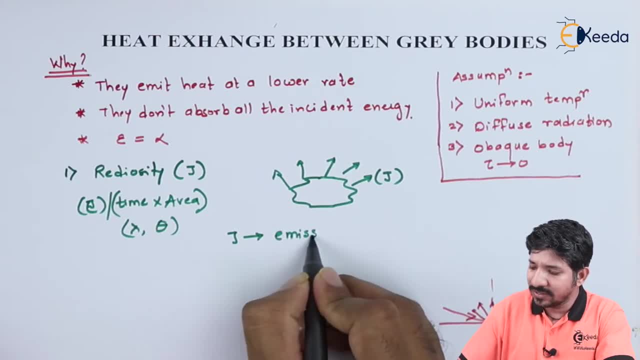 One is the emissivity, or the emission Of the given body, which is kept at some temperature, T. Now this since the value of T itself is higher than the absolute value, or let's say 0 Kelvin. So this body is going to emit some amount of radiation. 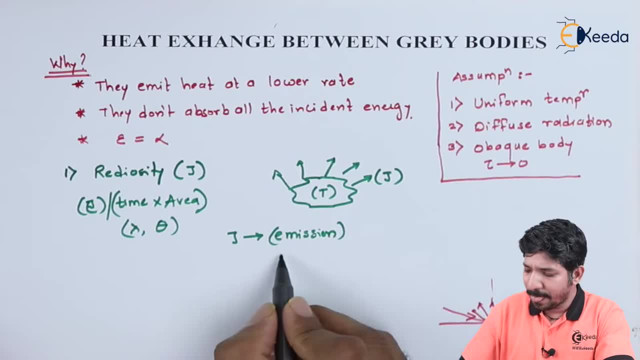 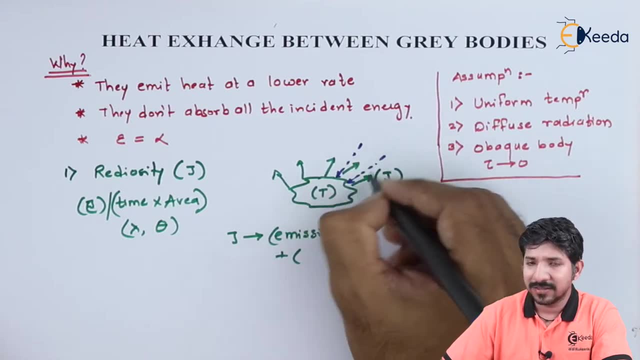 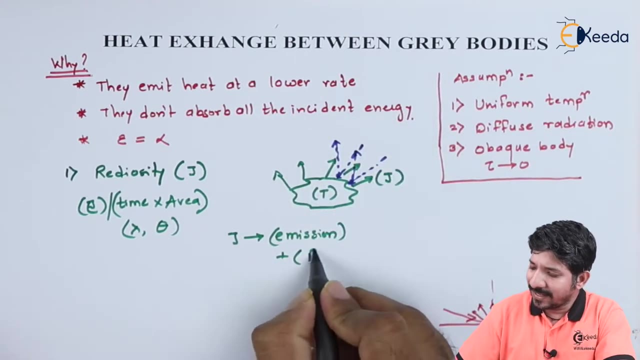 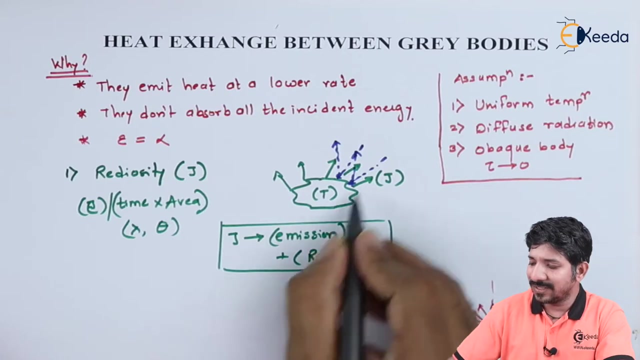 So that we are going to call as some emission Plus. now there is a possibility that from other body some radiation may come onto this surface and with that some amount of energy is also reflected. So basically I can call this as reflections. So the amount of energy that is radiating can have two aspects. 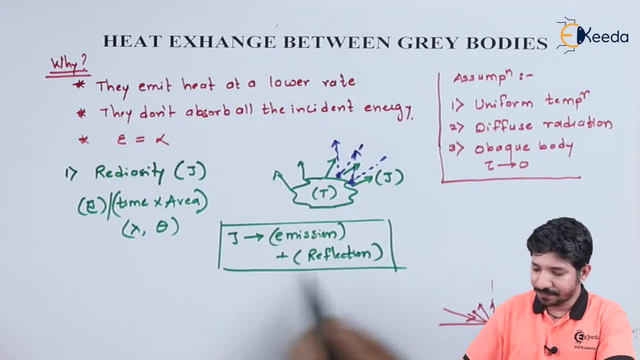 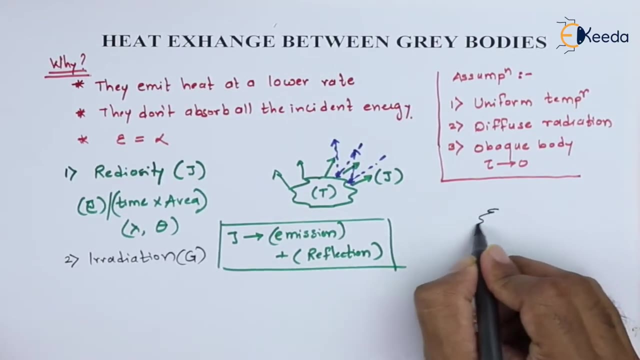 One is the emission of its own body and the other one is reflections. Similarly, the second one is irradiation. We call this as G. Now what is irradiation? G? It is the amount of energy that is coming onto the surface from the other body. 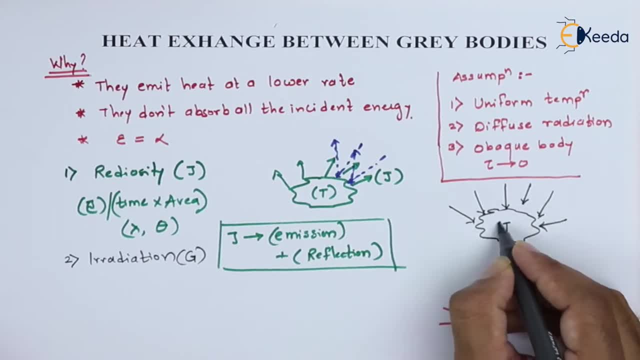 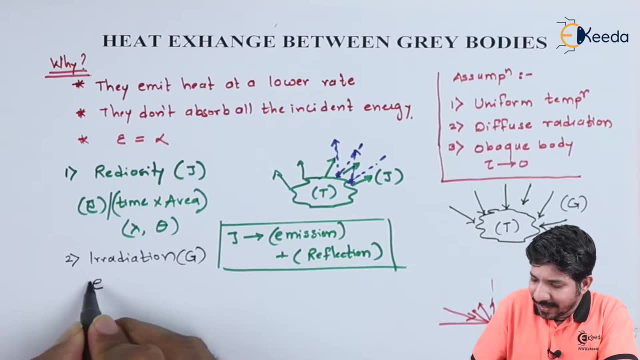 Now what amount of radiations are coming onto the surface which is kept at, again, temperature T? Now this is indicated by irradiation. Again, it is simply the amount of radiant energy coming onto the surface per unit time, per unit area for a given wavelength in a hemispherical direction. 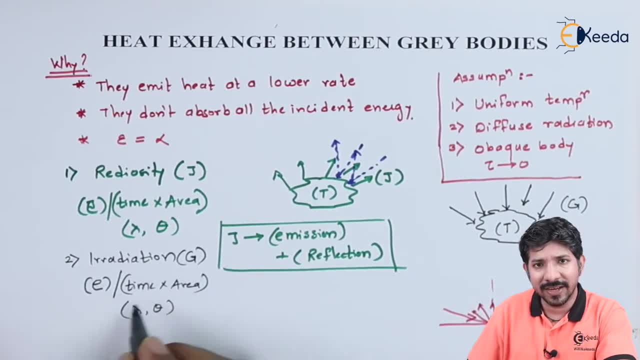 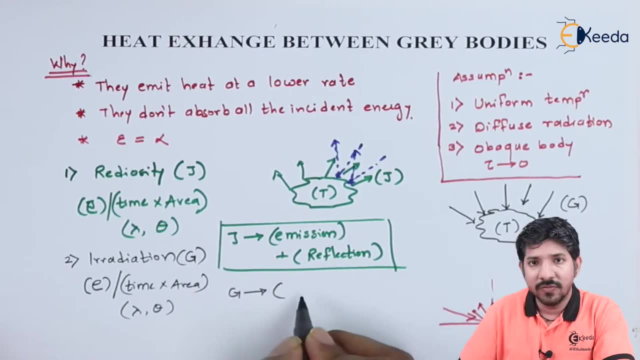 Now these four parameters one need to consider while analyzing any radiation problem. So for this also we can say that the amount of radiation itself can be the reflections of others, Plus the amount of energy That is getting reflected from the other body. So anyway, we will not discuss about this right now. 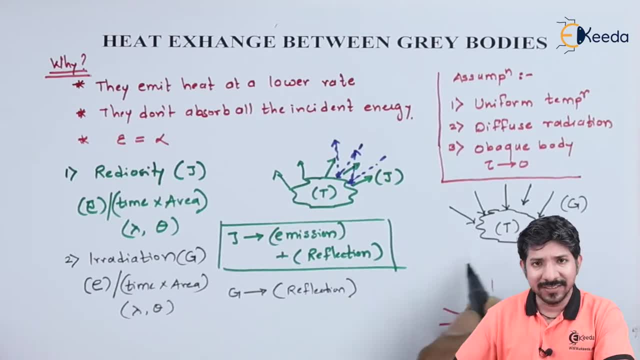 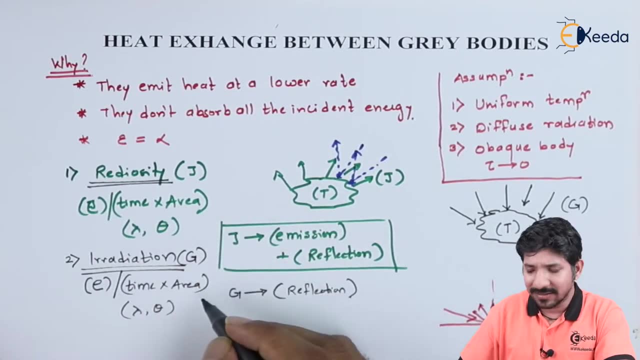 So let us keep it for the further discussion. Now just understand what is, what do you mean by the radiosity and what do you mean by the irradiation? And once we have understood this, we can go further. for the analysis of a gray body. 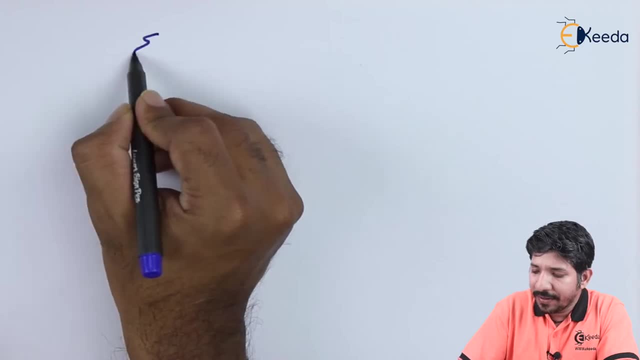 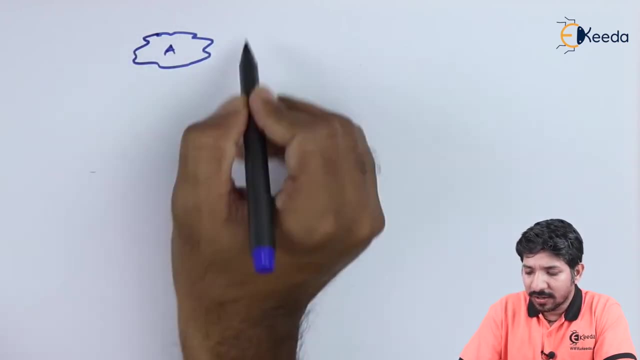 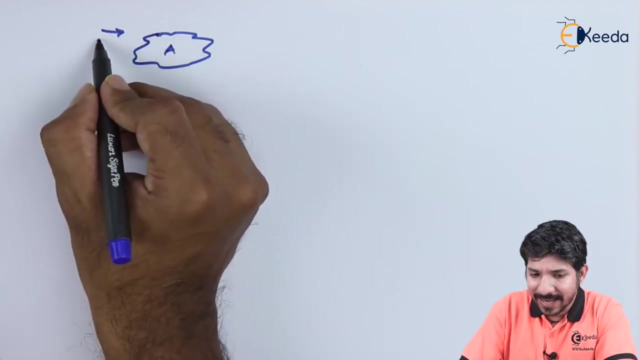 Now we can take a case of a gray body. Let's say this is a gray body, Now the radiations are coming from this, Or the radiations may come from this, other surfaces, Okay, so let us call that irradiation as G, and then obviously, 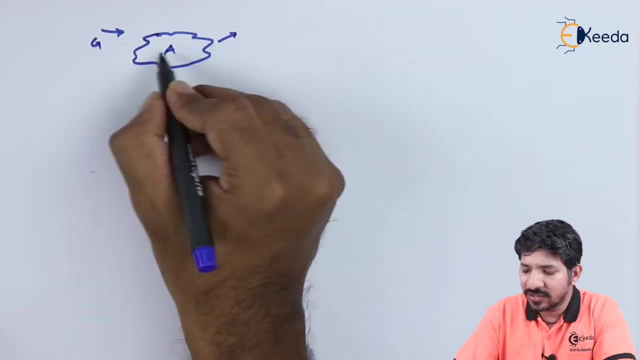 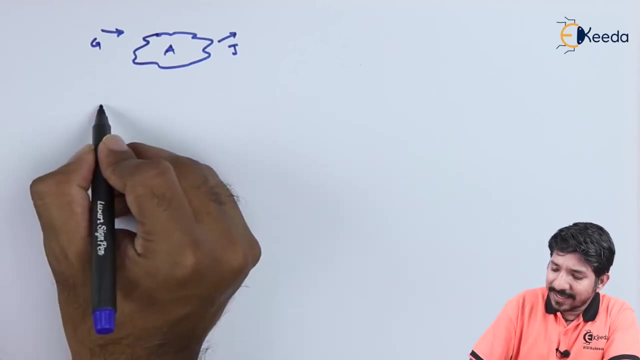 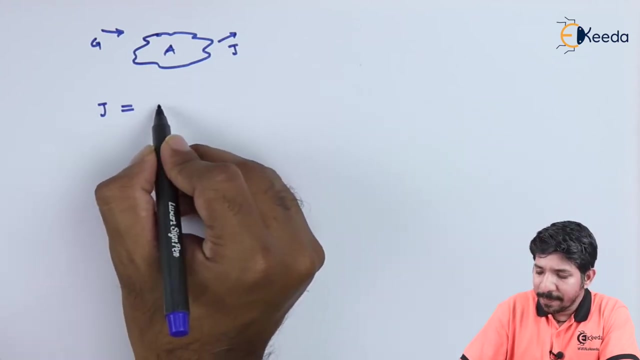 Some radio city is also associated with the same body. Let us call that J. Now we can have the expression about. the radio city means the amount of energy that is getting radiated. as I've told you before, This will be The reflections. 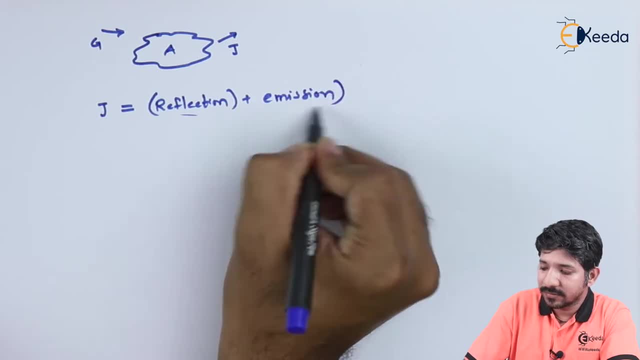 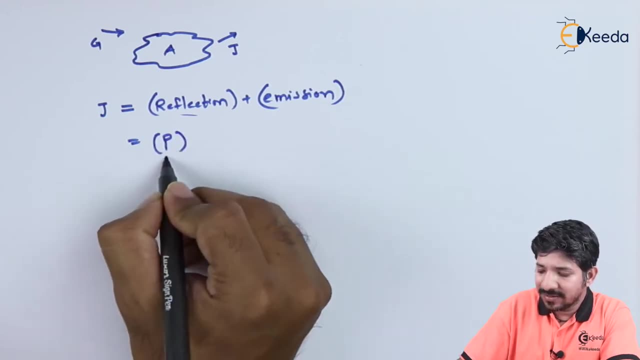 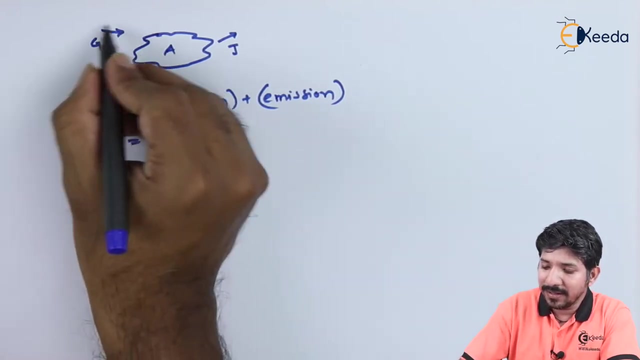 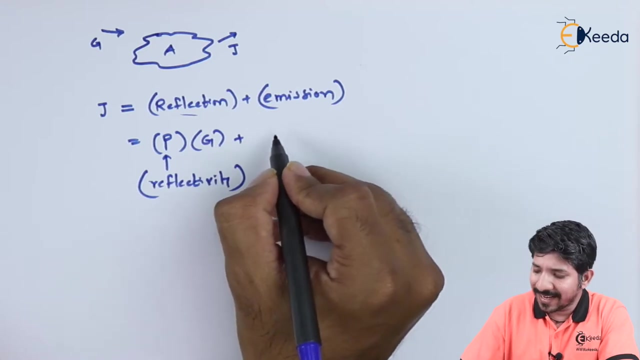 Plus the emission, Now the reflections. obviously this will depend on the reflectivity of a given body. This is the reflectivity Multiply by the amount of irradiation that is experienced by the body. And emission also is expressed As E. Now this is given by the emissivity: E into the emission in case of a black body. 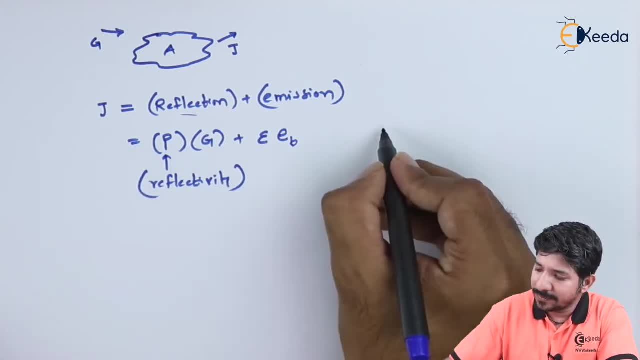 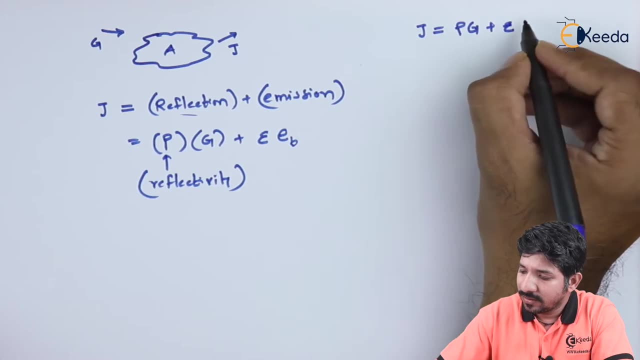 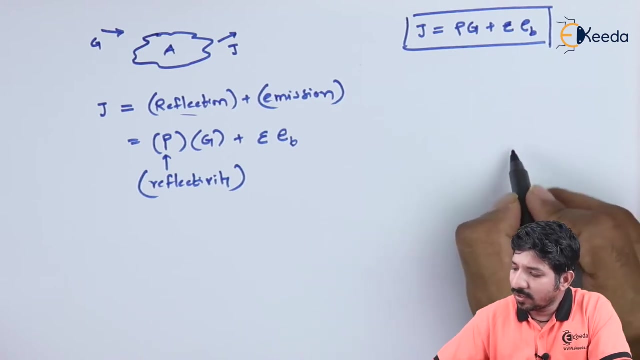 So basically I can write down the expression for J. Let me write it here As: rho into G plus The emissivity into EB. Now let us understand what we have done For writing the expression for. So if suppose some amount of energy, Q is coming. 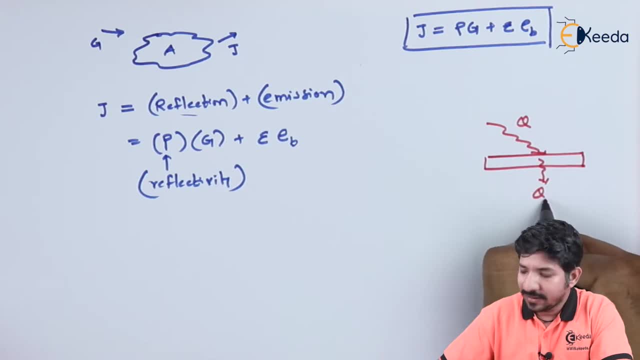 Some is getting, let's say, transmitted, some is getting absorbed- So let us call this QA- and some is getting reflected, QR. Now, from this we have said that there is something called the reflectivity, which is nothing but the energy that is reflected upon the total energy. 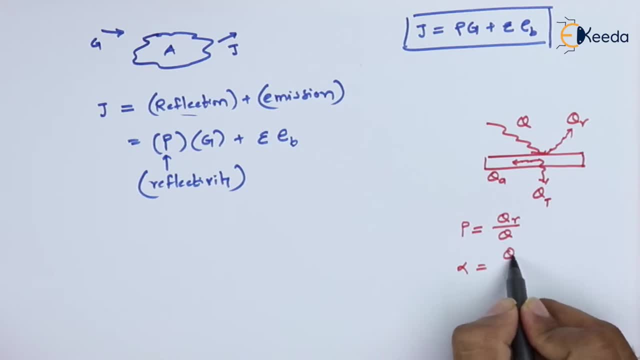 Then there is something called the absorptivity, which is the amount of Energy that is absorbed upon the total amount of energy that is incident on the given given surface, And then There is something called the transmissivity, which is the amount of energy that is transmitted upon the actual energy. 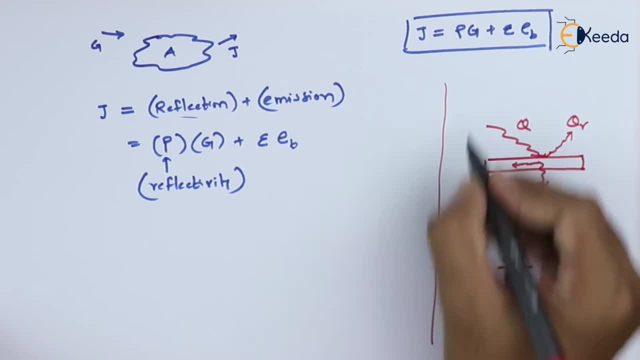 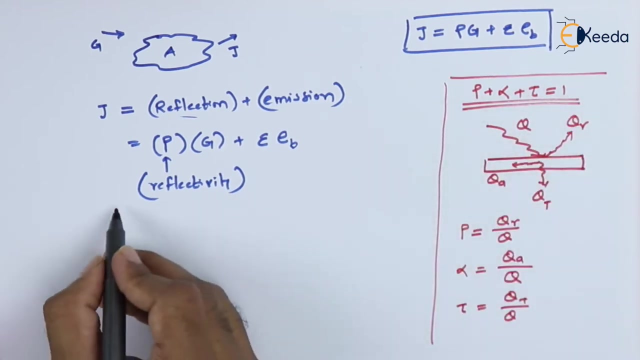 So from these I can make out that addition of rho, that is, the reflectivity plus absorptivity plus the transmissibility, Should be one. We have done this before. This is simply a recap. Now we know that for gray body. 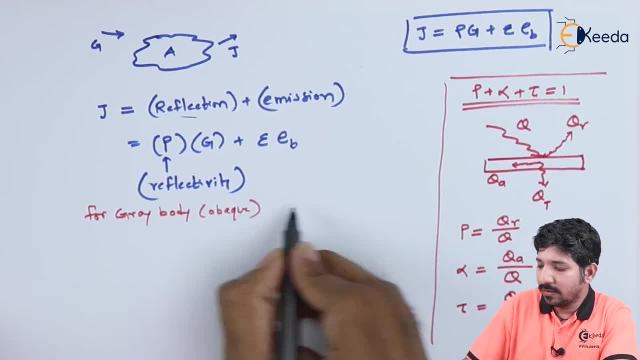 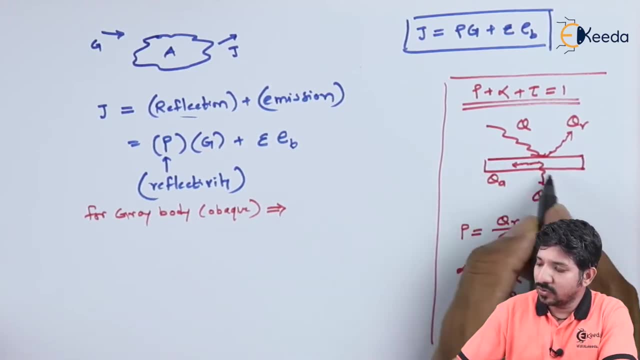 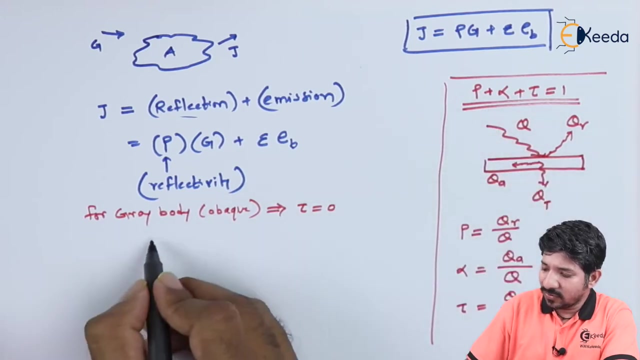 Which we have assumed as opaque. I can write down that for opaque body the value of transmissibility: there is no heat that will get transmitted. So means what: the tau has to be zero. So from this I can write down: rho plus Alpha has to be one. 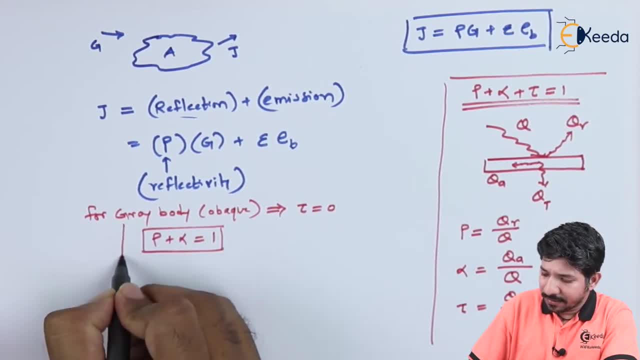 That is one thing. and for gray body, We know that alpha is same as emissivity. That is, for a given gray body, the value of absorptivity is same as the value of emissivity. Now, this is strictly given only for the gray bodies. 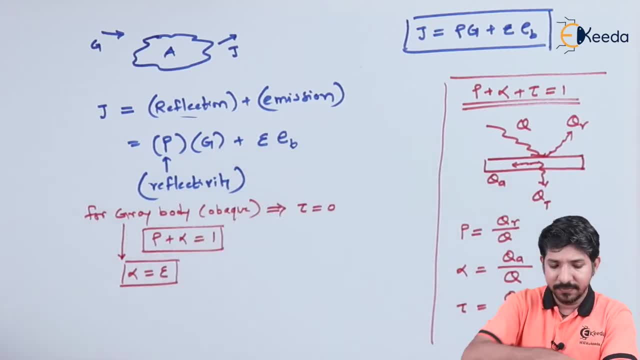 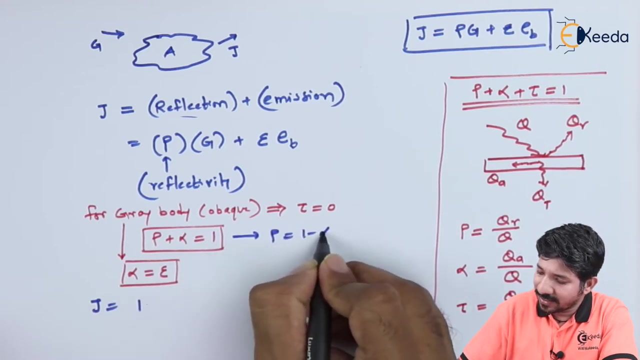 Now, with this thing in our mind, I can write down the expression. I can write this expression as J is equal to. Now, instead of this rho, I can write this as one minus alpha. So I can write this rho as one minus alpha. and then, instead of alpha, I can write this as one minus emissivity. 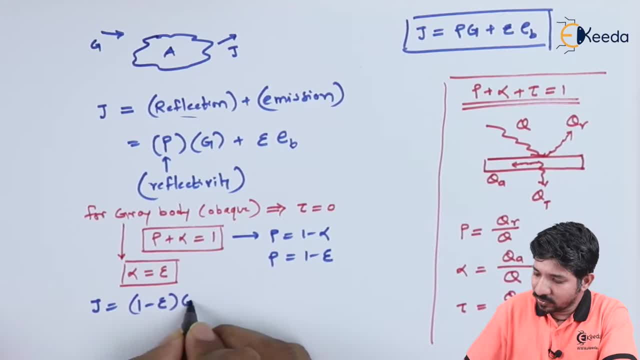 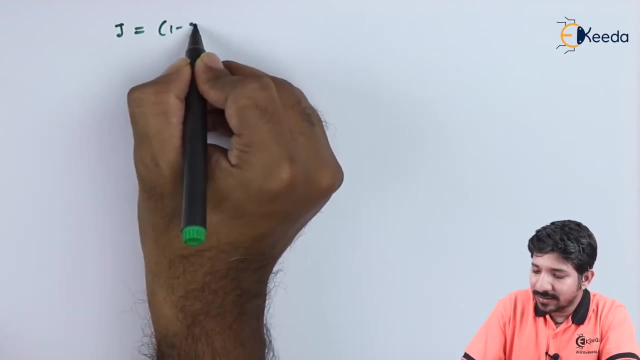 So rho itself can be written as one minus emissivity into G plus emissivity into EB. Now from this we can write down the expression for J. So let us write down the expression for J. The previous expression was: J is equal to one minus emissivity into G plus emissivity into EB. 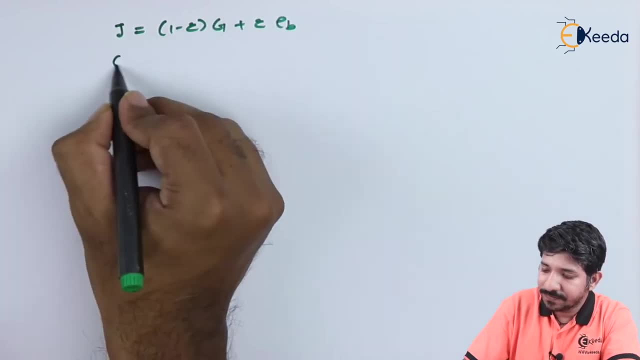 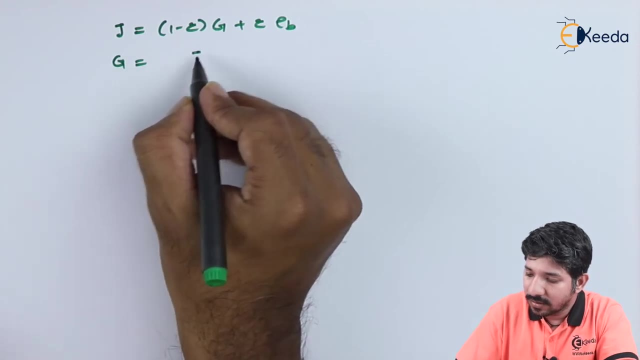 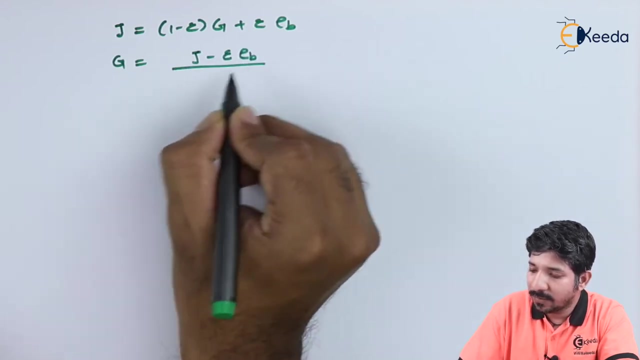 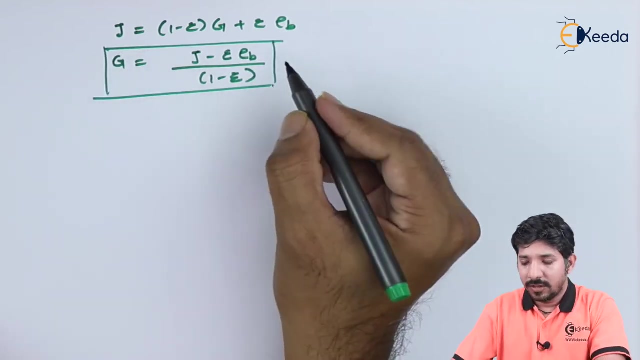 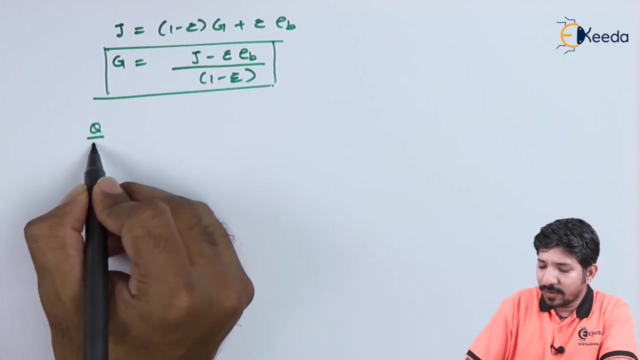 Now let us express everything in terms of G. So G is written as: J minus emissivity into EB upon one minus One minus emissivity. Now, when we are talking about heat transfer from two gray bodies, We can write down the amount of heat transfer per unit area. in that case can be written as: 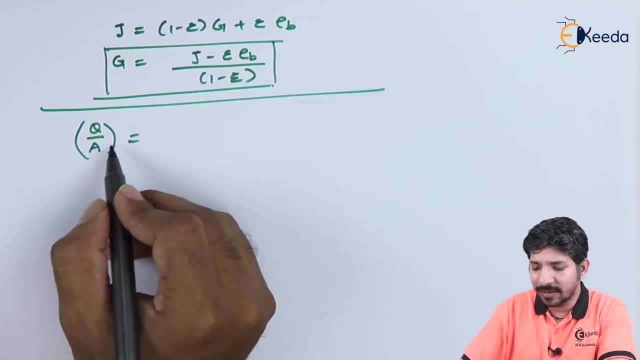 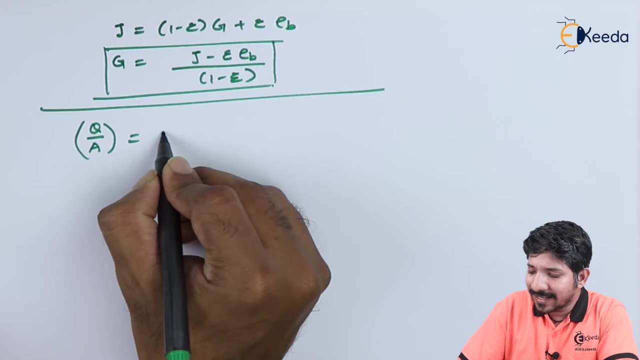 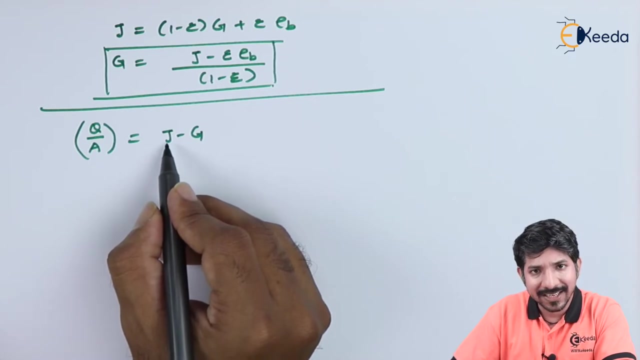 Now again, this is simply written for the heat transfer. in case of two gray bodies, It can be easily written as: So the amount of heat transfer per unit area can be easily written as J minus G. Now, what is J here? Now, here, J is nothing but the amount of irradiation that is coming into the surface upon the radiosity. 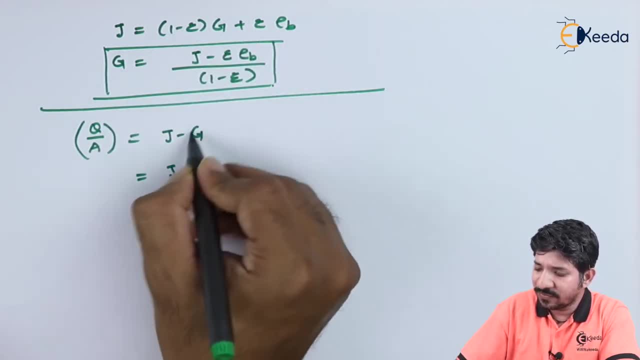 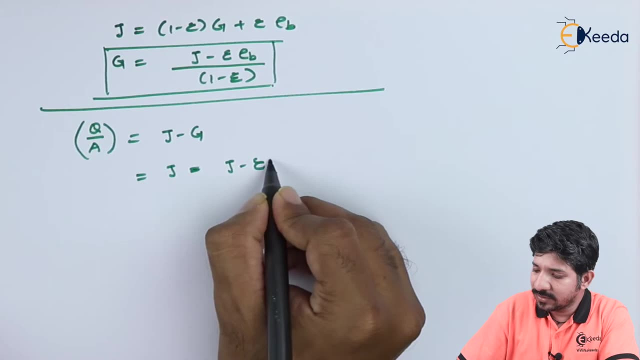 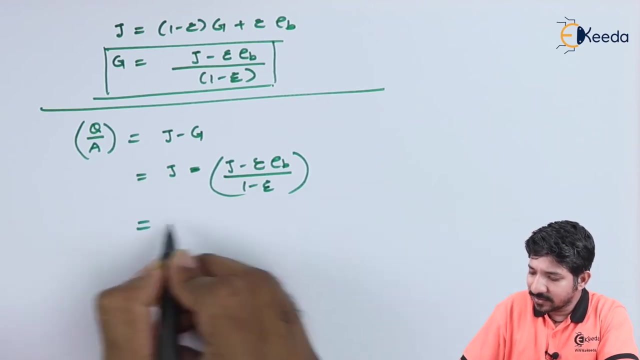 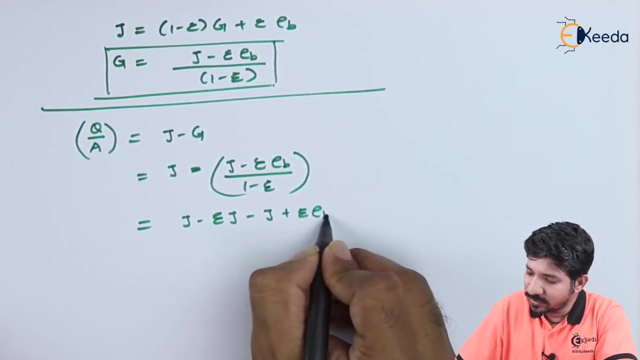 So now let us put the expression for G So this J minus, so emissivity EB upon one minus emissivity. Now, if I rearrange the terms, I can write this as J minus emissivity Into J minus J plus emissivity into EB upon one minus emissivity. 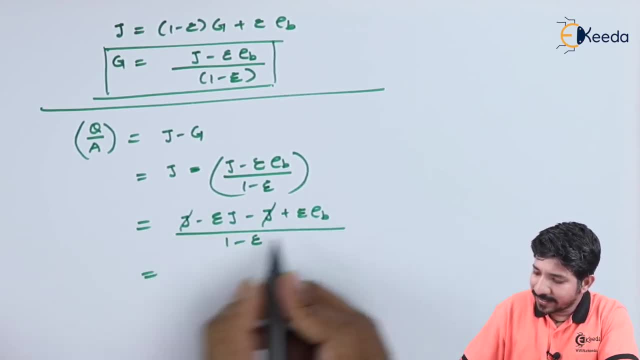 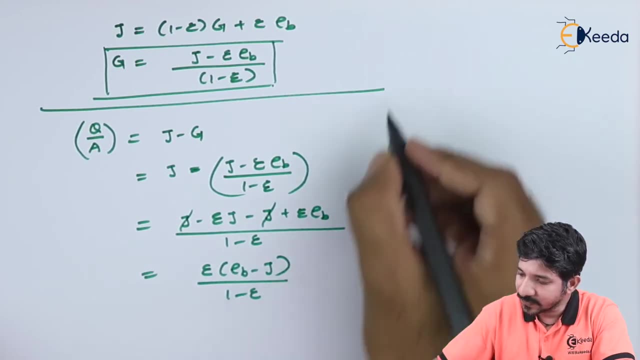 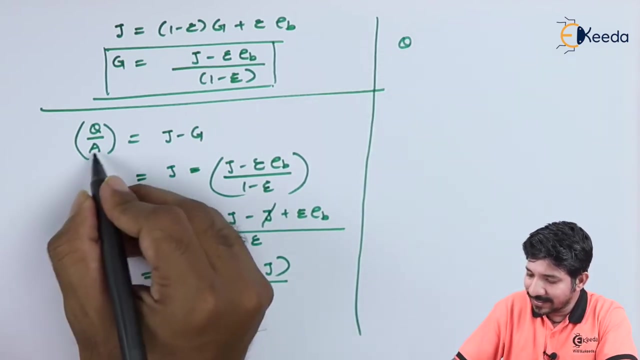 So I can cancel out this two terms And I can write this as emissivity in the bracket EB minus J upon one minus emissivity. So finally, I can write this as Q, or let me write it here itself: Q is equal to. I can take this A to the other side. 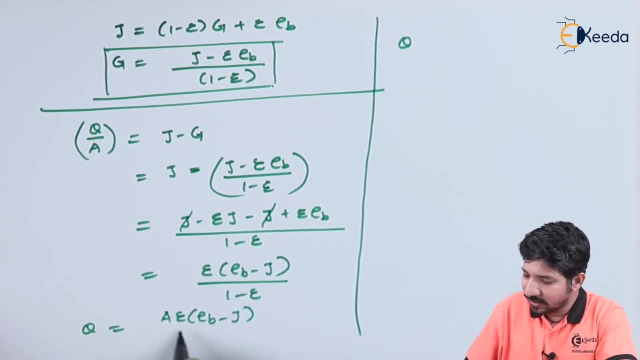 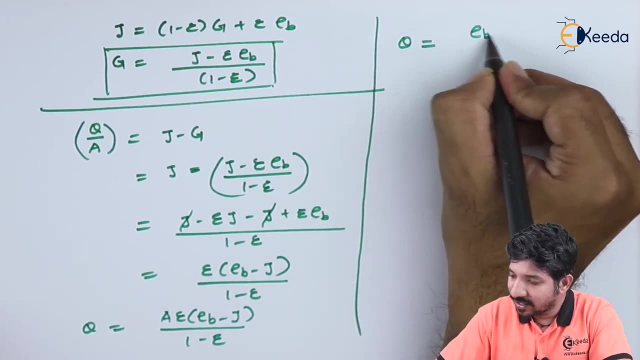 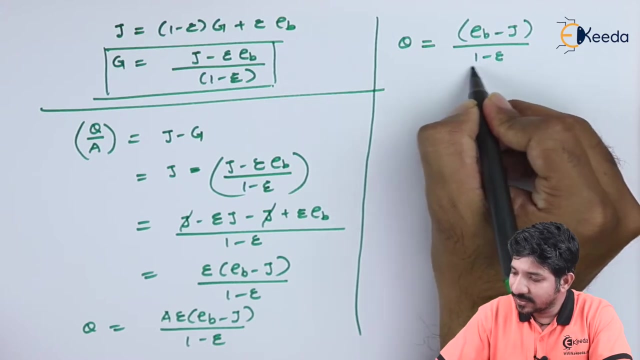 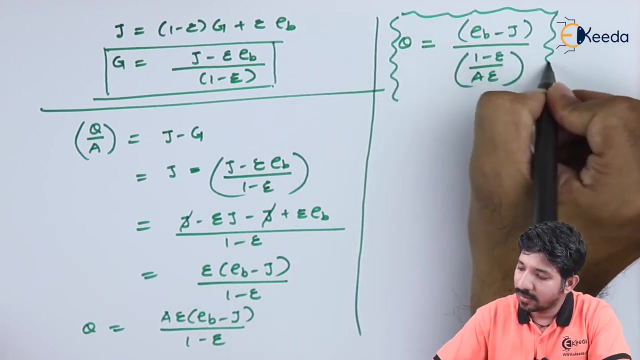 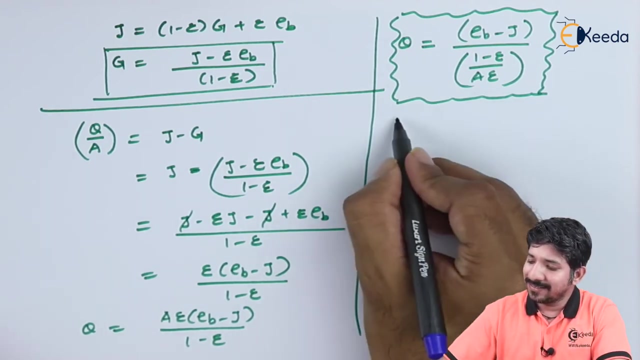 That is A into emissivity, EB minus J, One minus emissivity. Now I can write this Q as EB minus J upon one minus emissivity upon A into emissivity. Now this is one of the important expression that we have got Now here. I can write this in the electrical analogy: 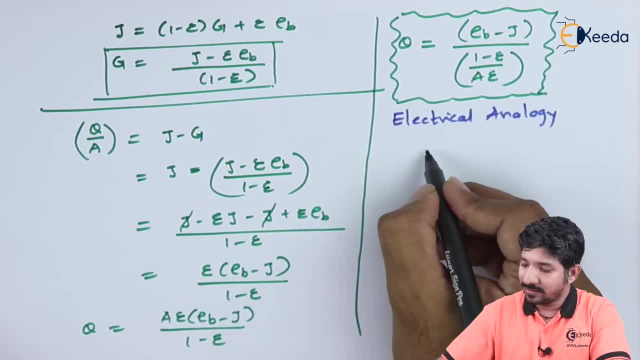 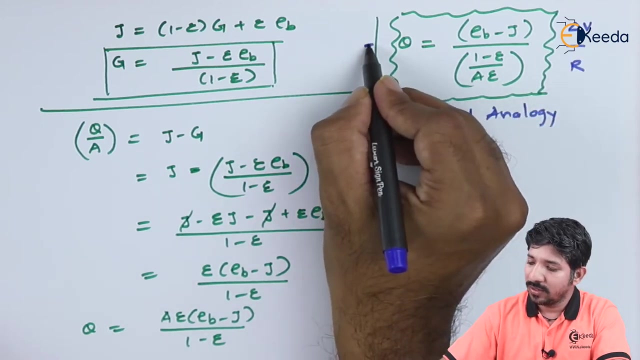 Which is, I hope you know that V is directly proportional to I, So according to that, we can write this: as this is nothing but the delta V, And this is corresponding to R and this is corresponding to the current I. So let us draw the diagram for the same. 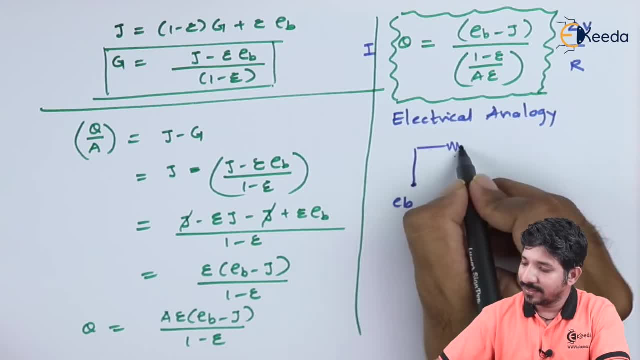 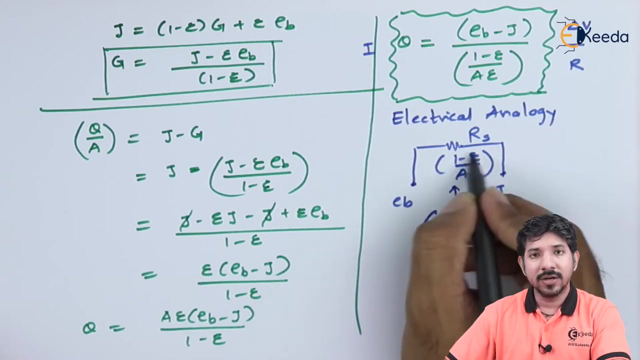 So I can indicate this as, let us say, EB, some resistance and then J. Now this resistance is given by one minus emissivity upon area into emissivity. Now this they call, as this is the resistance. They call this resistance as surface resistance. So this is one of the resistance offered for the radiation transfer from two gray bodies. 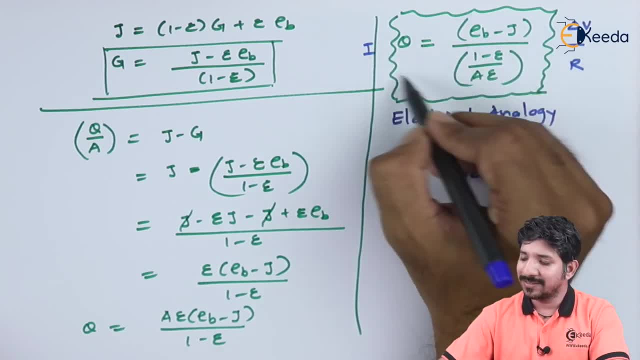 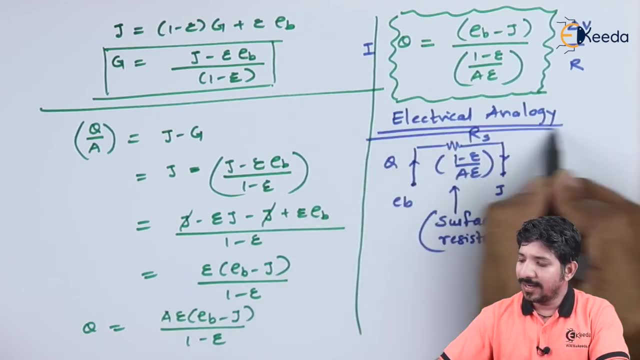 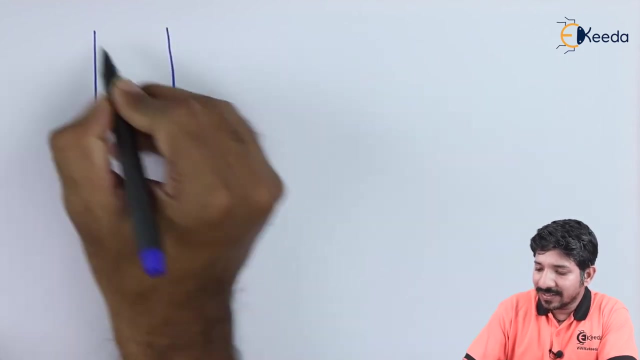 So they call this as the surface resistance, and the expression is given something like this: So where the heat transfer is given by Q itself. Now, this is basically the electrical analogy given for this case. Similarly, we can also consider two surfaces. Let us call this surface one. 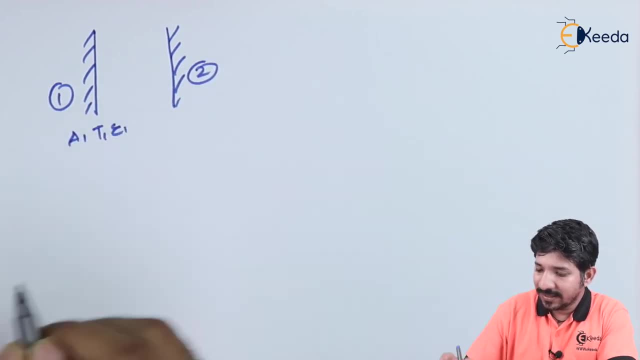 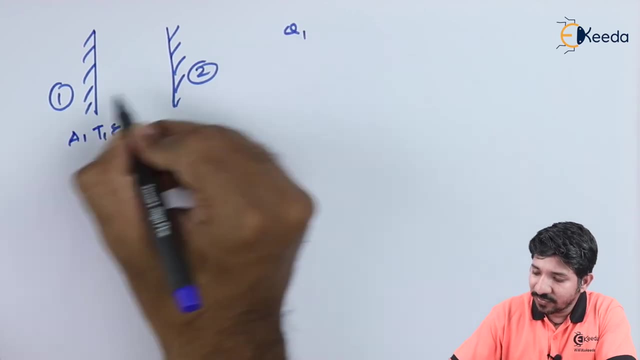 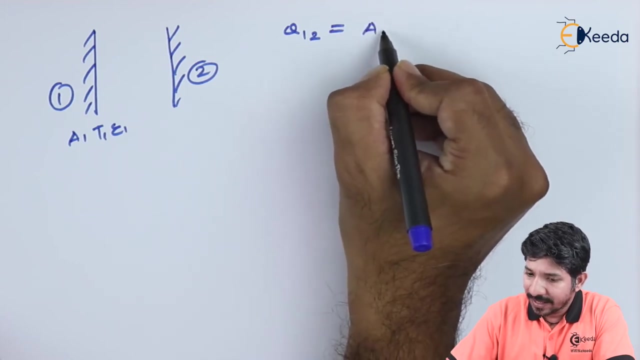 This is two. This is kept at A1, T1 and emissivity one. Now, in this case, I can write down the amount of heat Q that is transferred from surface one to two. As we have seen this previously, It can be given as A1 into F1 to 2 into J. 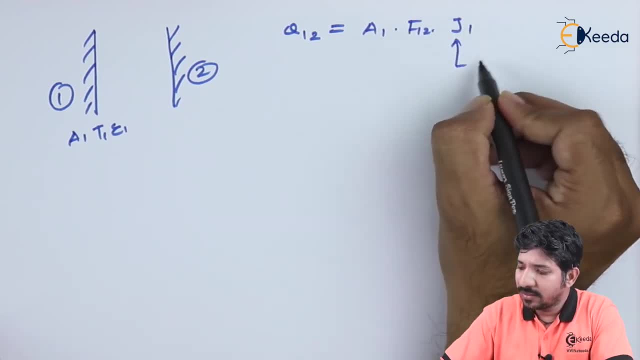 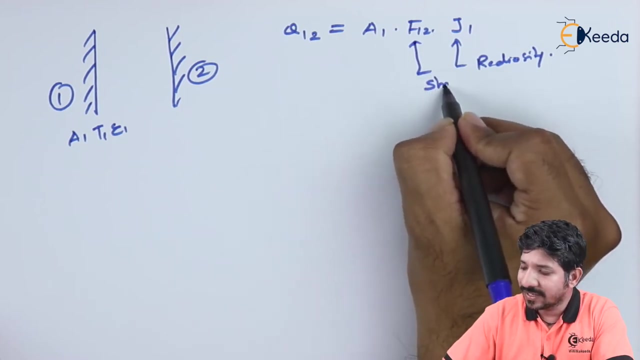 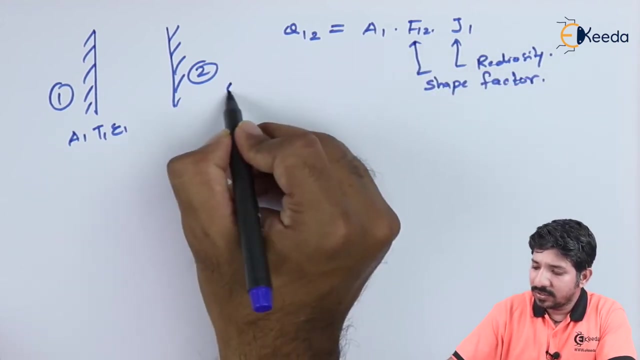 Now where J1 is nothing but the irradiation or the radio city, in case of Q1 to 2.. And F1 to 2 is nothing but the shape factor. So the same way I can write down for Q2 to 1, which is A2, F2 to 1 into J2.. 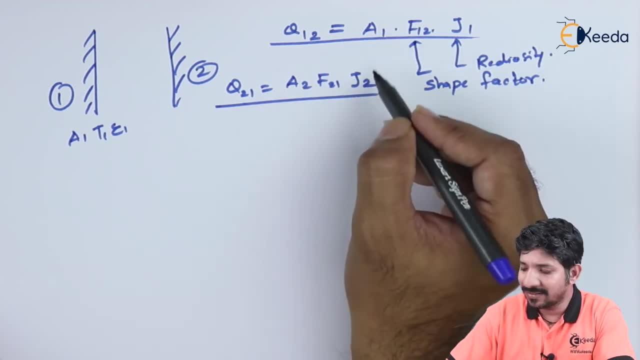 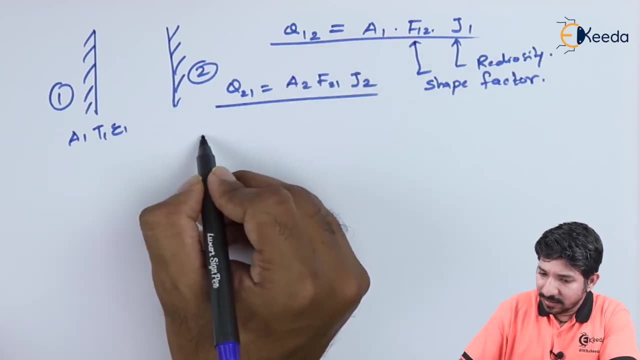 Now these two expressions can be easily understood, If you understand. what do you mean by the shape factor, which we have previously discussed about. Now the net heat, That is, the value of heat transfer, either from 1 to 2 or from 2 to 1.. 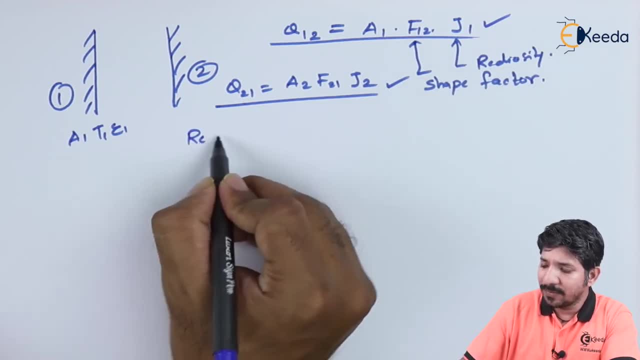 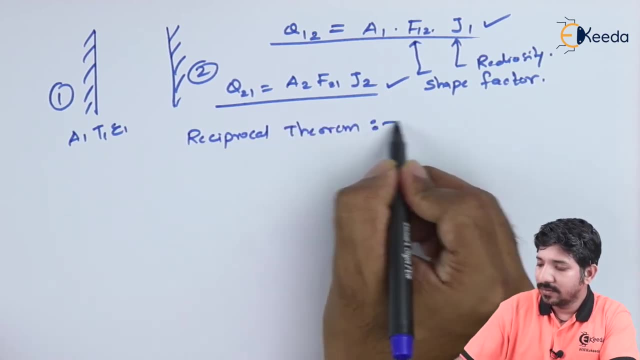 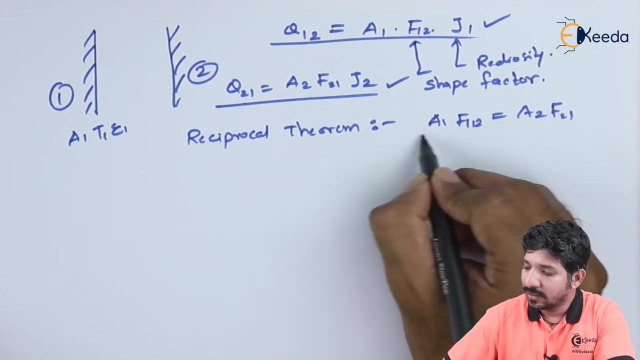 We can get with these two expressions, But there is something called the reciprocal theorem. Now, with this reciprocal theorem, We know that A1 into F1 to 2 is same as A2 into F2 to 1.. If this is the case, then what is the net change? 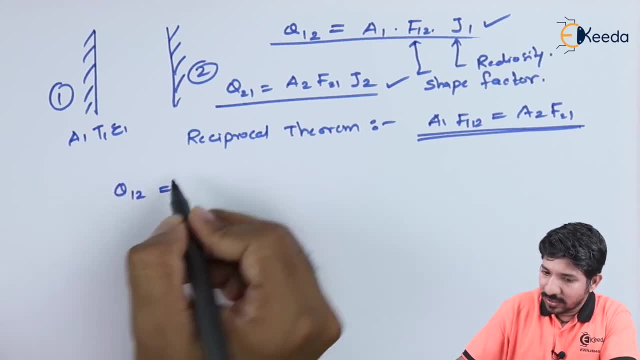 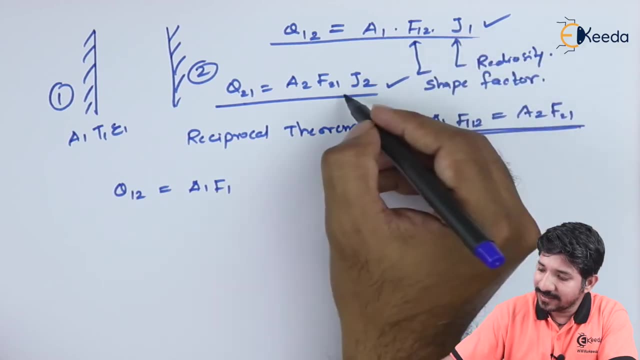 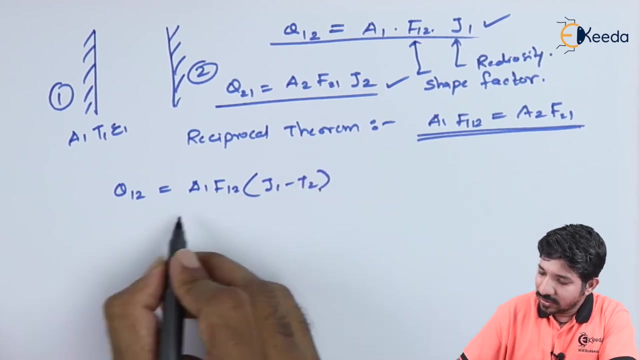 The net change here, that is, Q1 to 2, can be easily written as A1 into F1.. Now we are taking the net change here. I can write this F1 to 2 in the bracket J1 minus J2.. Now this is simply the expression here. I have rewritten it. 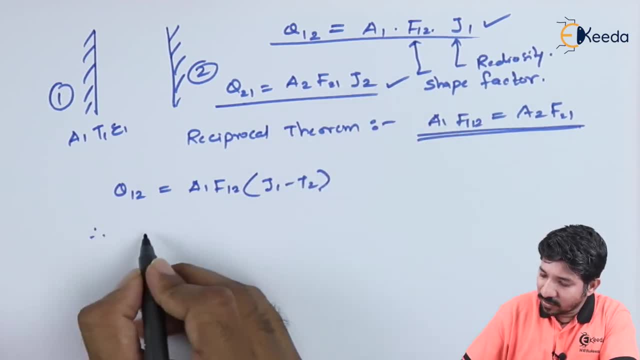 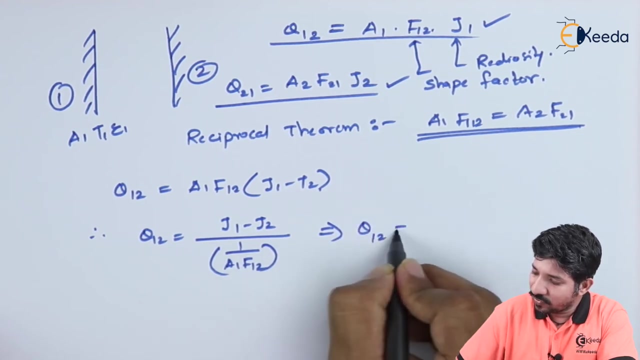 Now I can write down this in some other format: Q1 to 2 is J1 minus J2.. J1 minus J2 upon This I can write as 1 upon A1, F1 to 2.. Now this I can again write as Q1 to 2.. 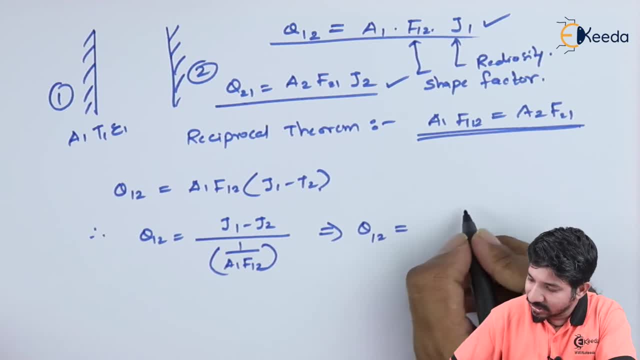 Now this J1 and J2 I can express in terms of the emissivity, And so this is basically the. So let me rewrite again: J1 minus J2 upon 1, upon A1, F1 to 2.. Now this A1, F1 to 2.. 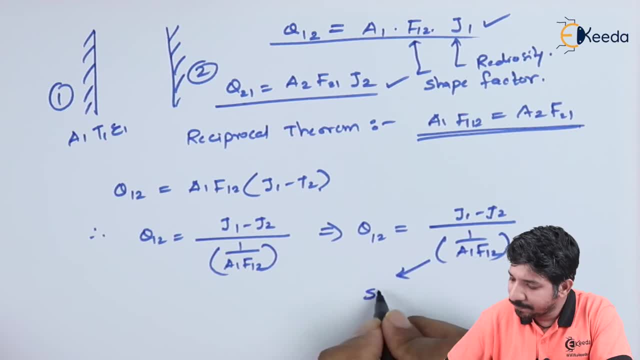 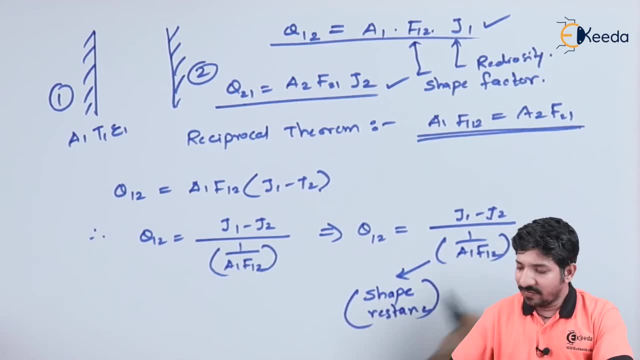 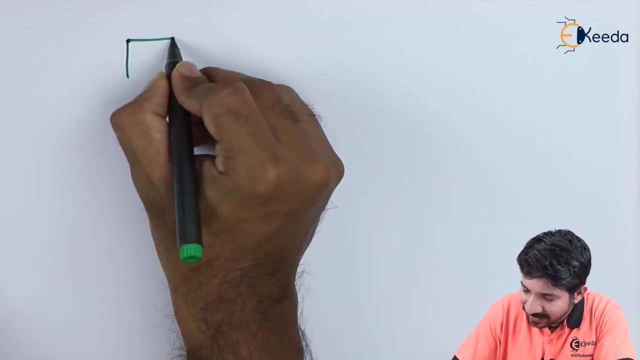 1 upon A1, F1 to 2 is nothing but the Shape resistance. Now, if I want to express both the resistance, So again, if I want to find out The amount of energy that is transferred from one body to another body. 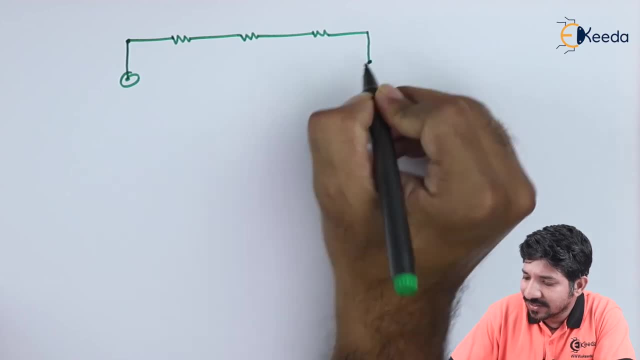 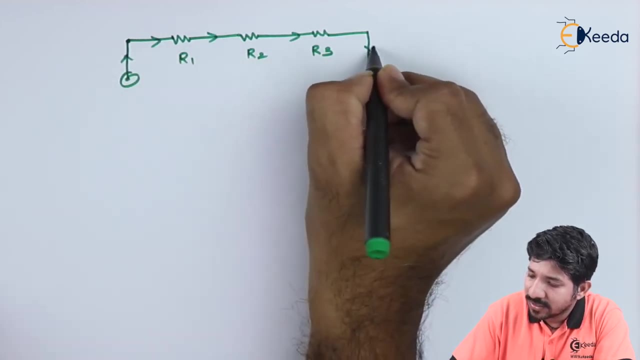 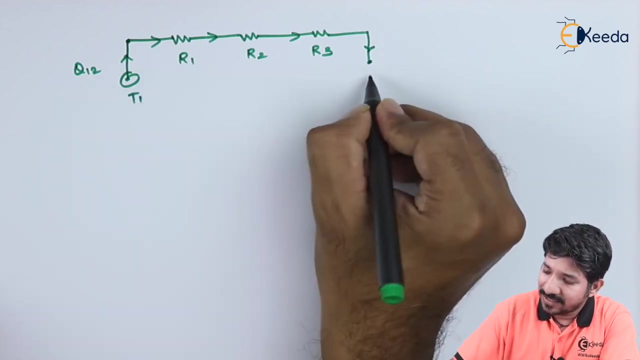 I will have to consider three distinct resistance. Let us call this R1, R2, R3.. So this is the heat transfer. This is, let us say, Q1 to 2.. Okay, So here I can write this as T1 and this is T2.. 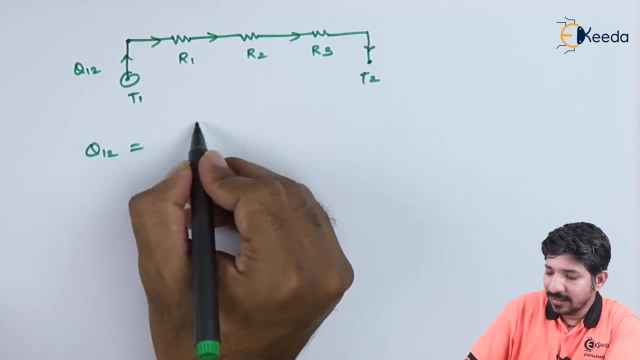 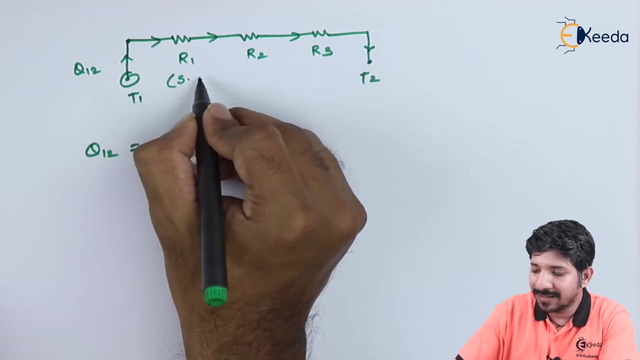 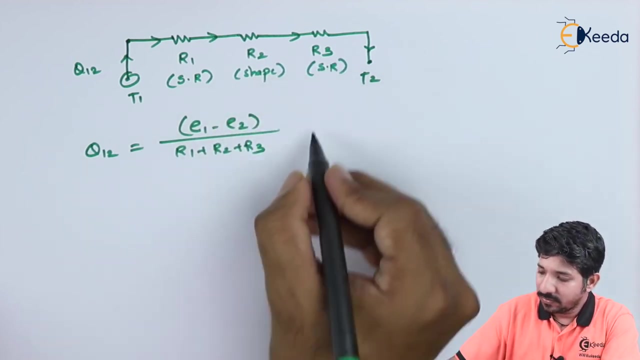 We have seen this before, that Q1 to 2 can be easily given out by the emissivity, That is, E1 minus E2.. Upon all the resistance Where this one represent the surface resistance. This is the shape resistance And again, this is the surface resistance. 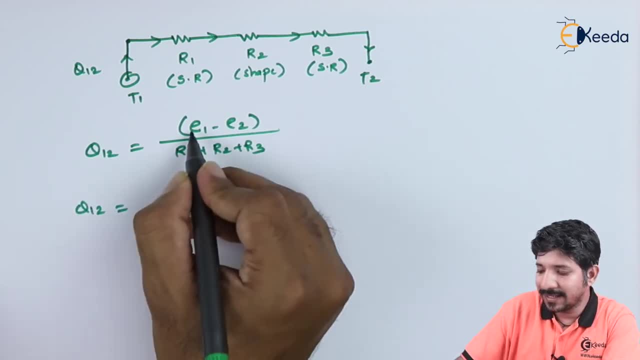 So let us rewrite the same. Q1 to 2 can be written as now. E1 and E2 can be by Stefan Boltzmann law. I can write this as: T1 raise to 4 minus T2 raise to 4.. 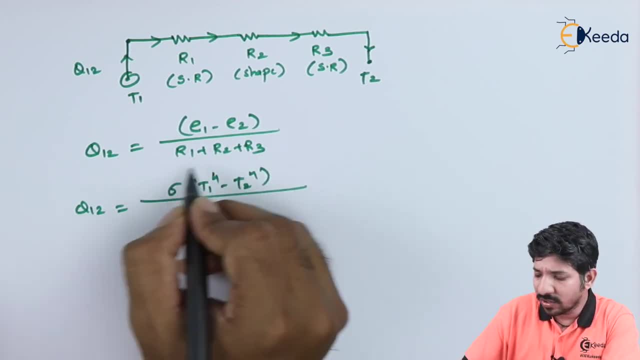 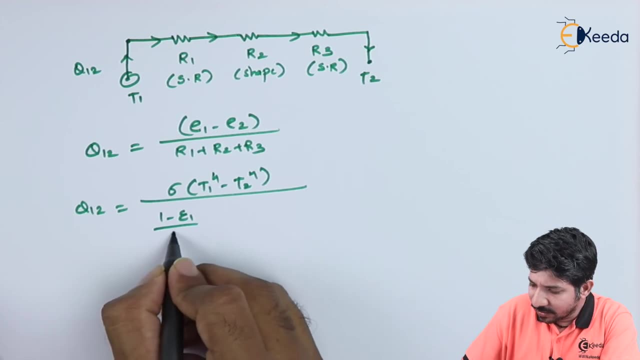 Now this is nothing but the Stefan Boltzmann constant upon. Let us write all the resistance. This will be 1 minus emissivity, 1 upon the emissivity, 1 into A1.. So this is what they call as the surface resistance. 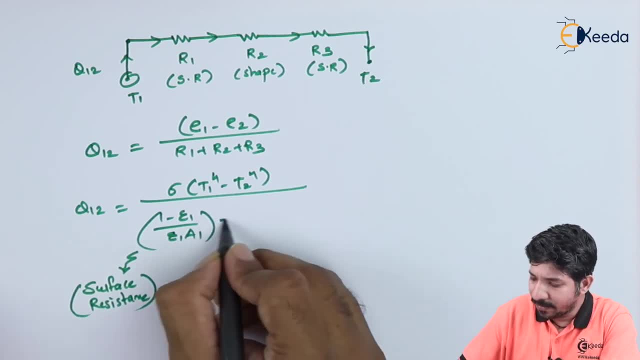 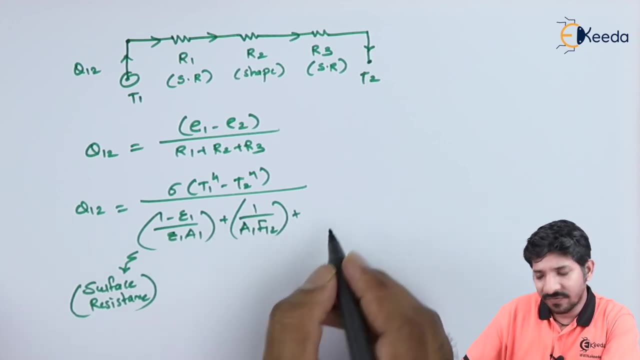 For surface 1 to surface 2, plus 1 upon A1, F1 to 2.. And this is again the surface resistance for 2 to 1.. So 1 minus emissivity 2 upon emissivity 2 into A2.. 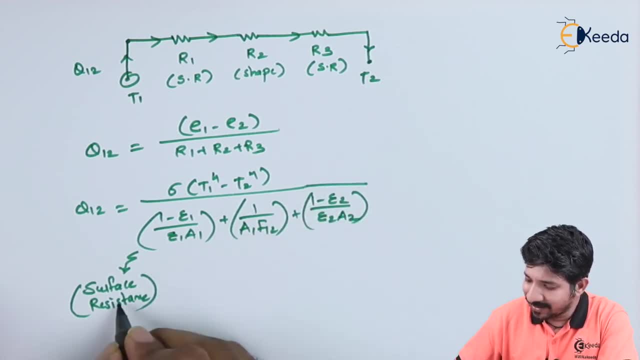 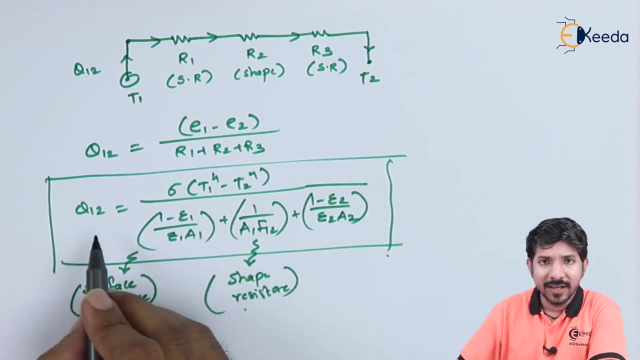 So I can write down that these two are basically the surface resistance And this one is shape resistance. So this way, basically, we have tried to figure it out. What is the value of heat transfer rate, Or the net heat transfer rate, in case of a radiation?